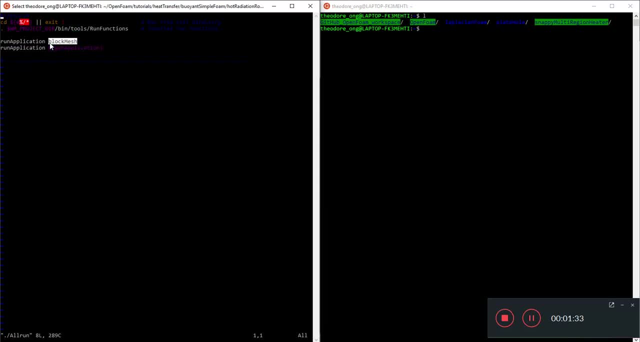 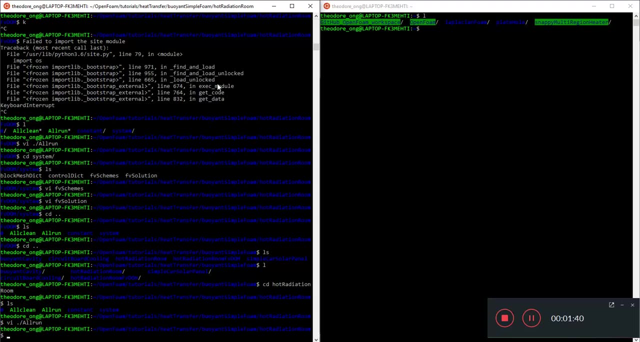 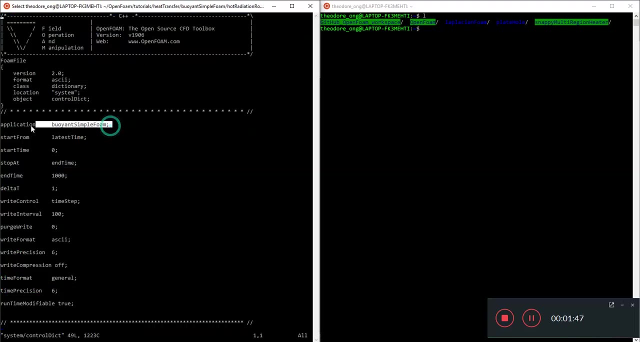 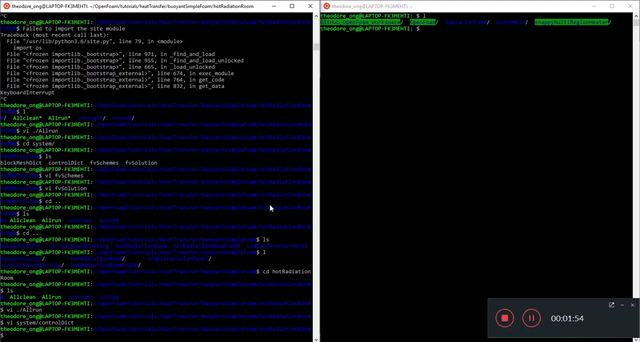 So this, this case is pretty simple. It's just running a block mesh and running the get application, which is buoyant, simple form If you look into the control dictionary. Okay. so where's the control dictionary? again? for those not so familiar, you should be familiar by now- But this is where the application is from: buoyant, simple form. All right. every time you see that get application, that's where you find it from, All right. so let's take a look at the zero directory, where we go find boundary condition. 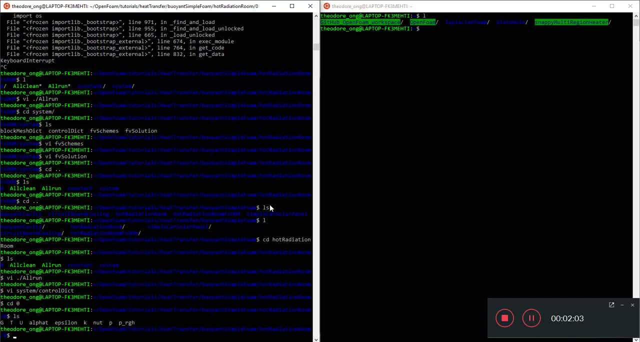 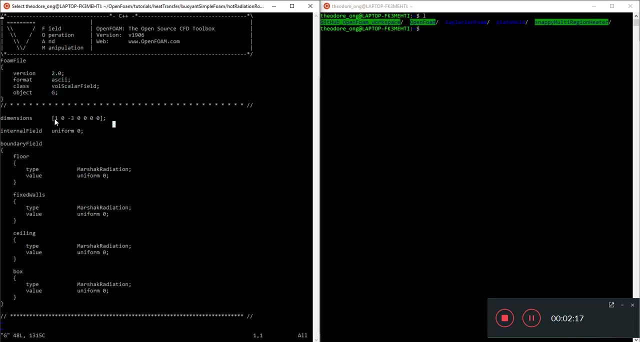 Okay so there's a GTU- blah, blah, blah, blah blah. we have discussed all of this before, except for this G term, So let's take a look at what is inside this G. Okay so it's a volume scalar field. the dimensions are one, zero and minus three, So that is some kind of- yeah, it looks like something to do with radiation. Okay so the bound: there's a. 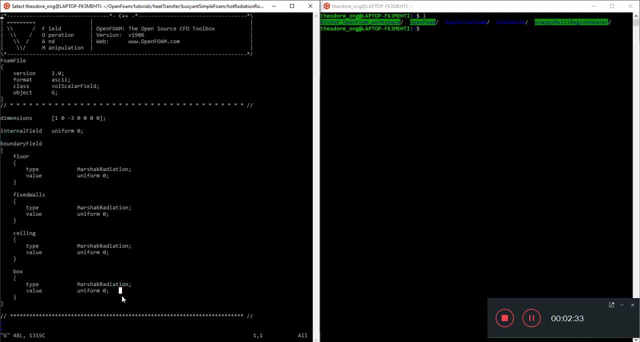 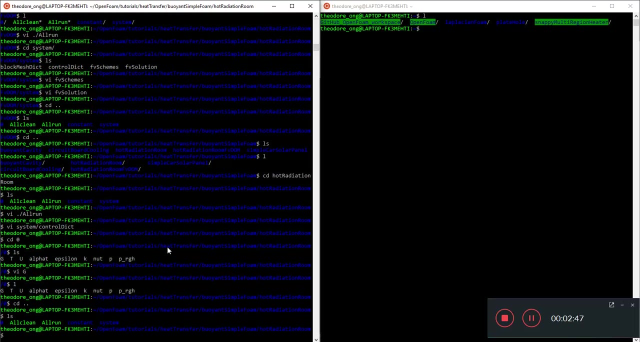 internal field of zero. boundary field of zero. Okay, so this? this looks like it has some something to do with the radiation. Okay, so in that sense, you need this extra little input file. All right, so we're just going to explore the rest and how it is different from, let's say, the convection case we were talking about earlier. So, all clean, we kind of know what it is. Let's take a look at the system directory. 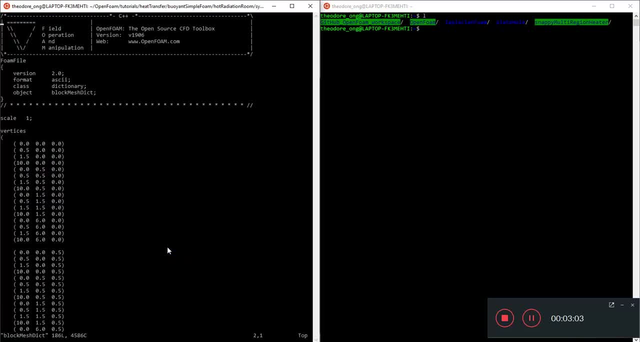 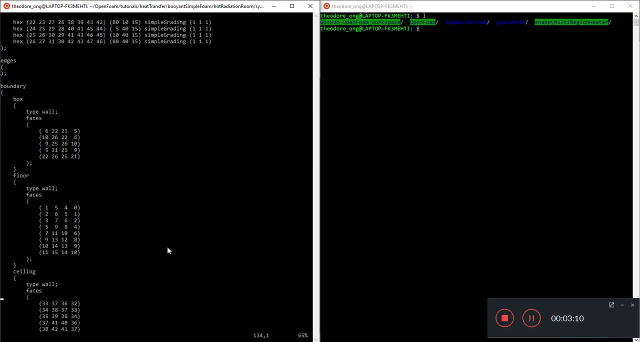 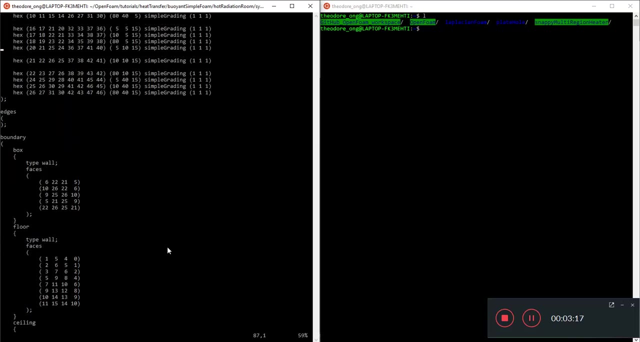 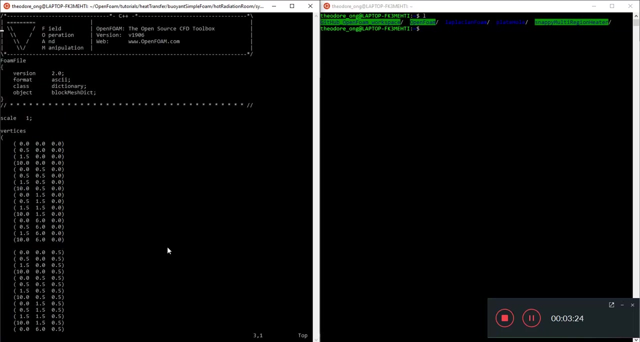 Let's look at block mesh to see what the geometry is like. So you'll see lots of vertices here Meaning to say: well, this is, this is pretty complex shit. as far as block mesh goes, Personally I wouldn't recommend writing block mesh like that. it'll give pretty much a headache. I'd rather use a snappy hex mesh using a some sort of computer aided design, so that you don't have to do. 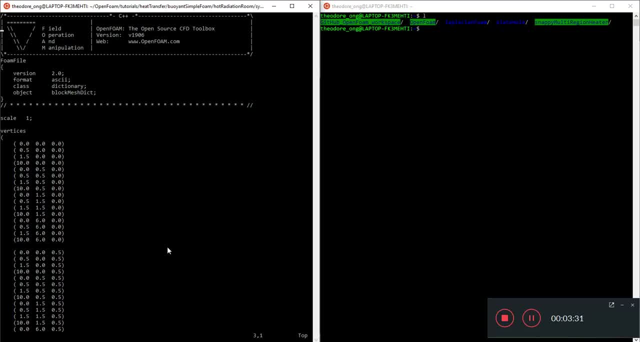 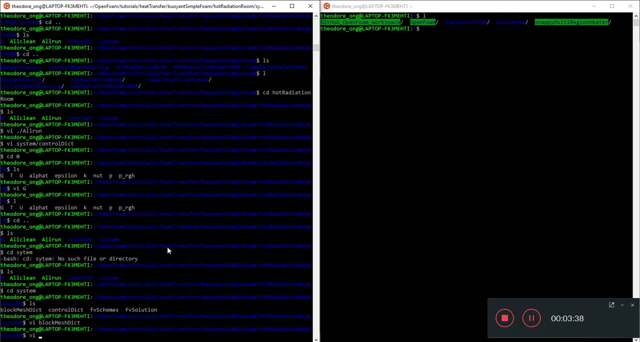 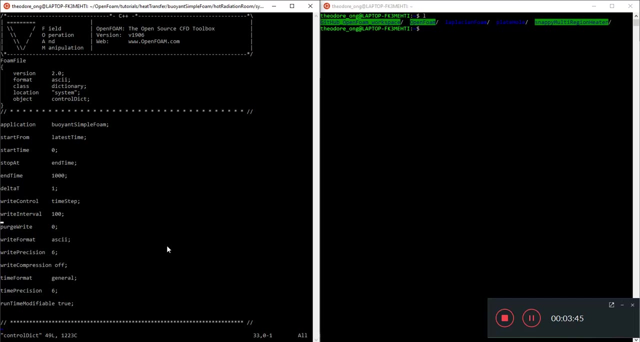 vertices point by point. It's really a big headache to go and write this out. But that is that. all right, That is that. Next thing we take a look at is the control dictionary. Okay, the application is born in simple form: blah, blah, blah. We have a write interval of 100, blah, blah, blah. Nothing, nothing too new here. Delta T can be 1 because it's a steady state solver. All right, so let's take a look at FV schemes. 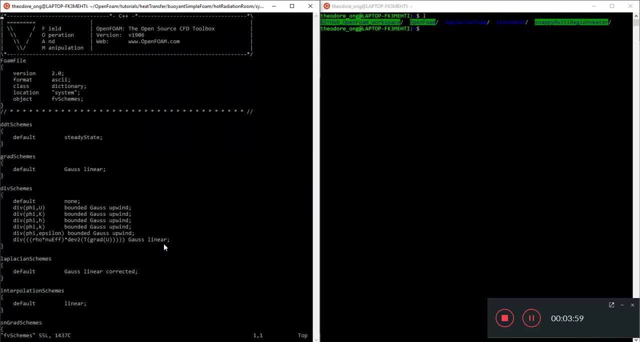 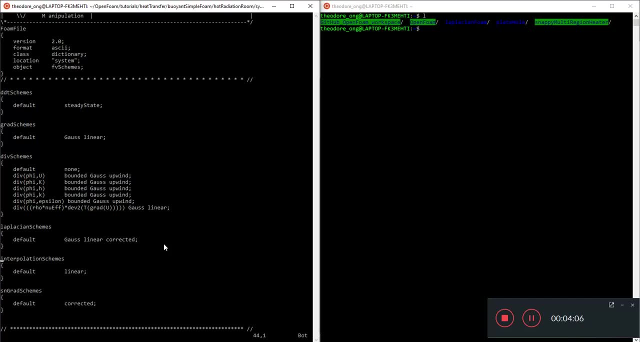 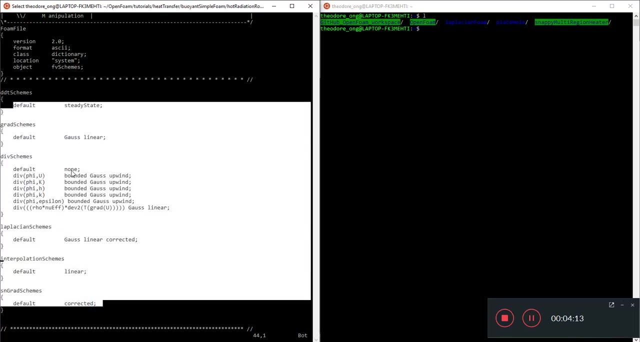 Okay, This is in case you want to copy and paste the file over or you want to. you have a geometry general of歸 file that you want to run Boyan simple form in. you've got to give the solver for boil simple foam, some inputs. So these are the inputs you need to give warm simple form. So yeah, it, it'll tell you: yes, all 70, 00. 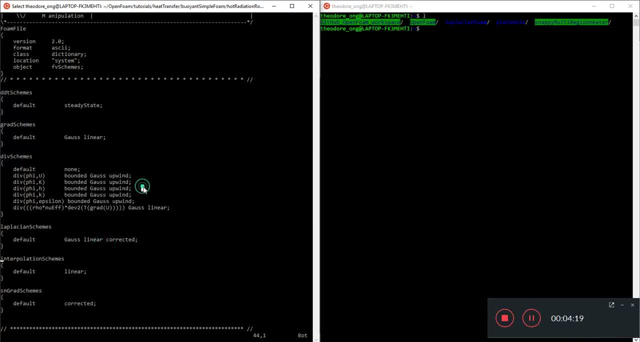 00 00 00 00 00 01. 10 00 00 0, 0. Mirror 7 00 00. the till for how do I solve this? divergence equations. Okay, so all these here. you'll need to tell you- Yes, you have to tell one simple form: How do I solve this? divergence equations? Okay, so, all these few. your need to tell this to some point of view. 9 00 00 00 00 00 00 00. *** apparently order. localizable verb. 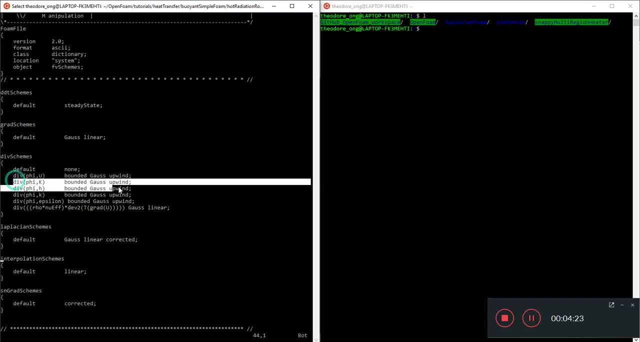 in simple form. how do I solve these divergence equations? so all these here you'll need to take note of if you want to pot it over. so these are all the inputs you need to give it. these are just input files. so DDT is a steady state, as you can see here. Gauss linear scheme. 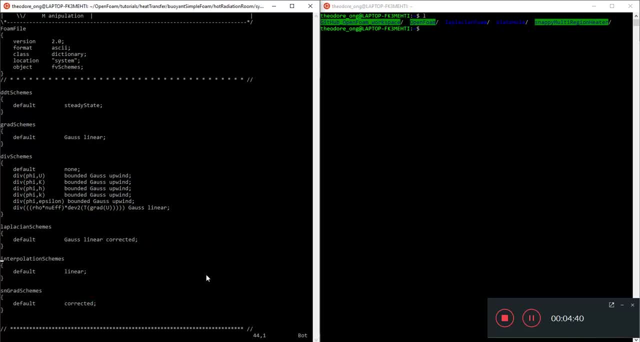 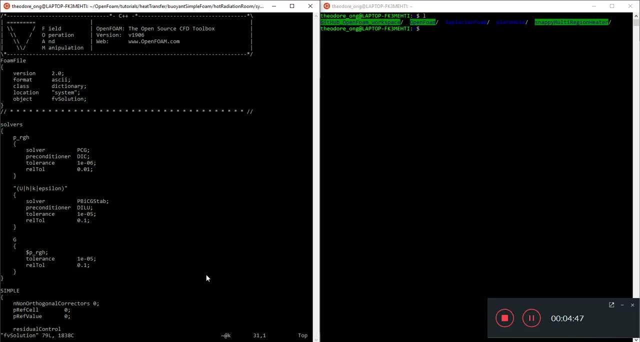 blah, blah blah. so nothing too new there. alright, let's go to FV solution and again we'll have some other inputs, and for UHK and Epsilon we'll have D solvers, P, rho, GH, D solvers. G will be D solvers. 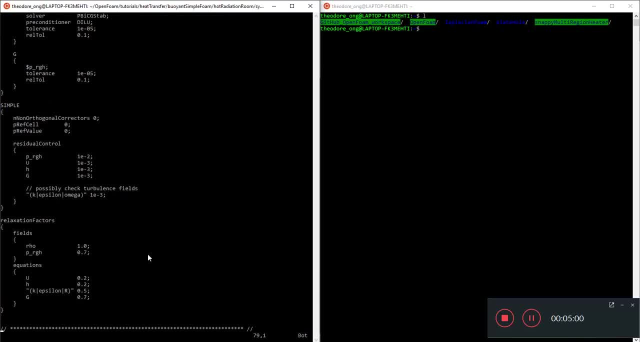 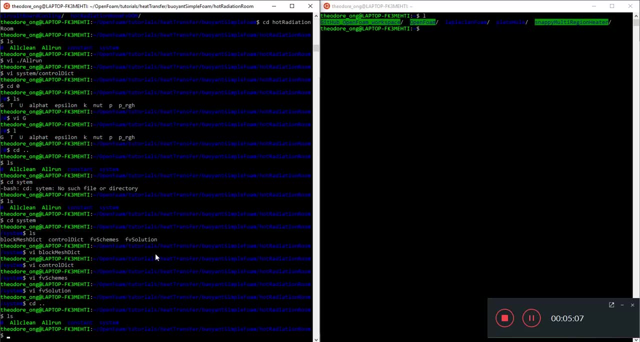 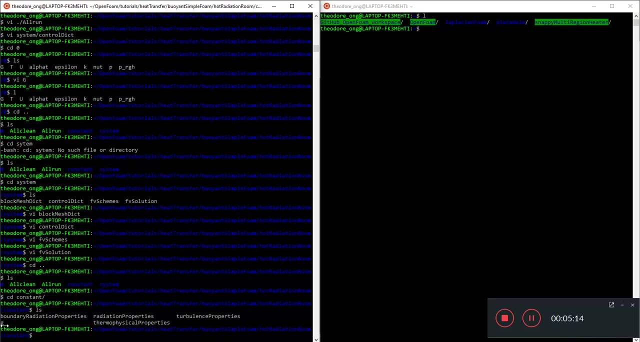 and G- remember this is a radiation thing, so we'll have all these factors in- gives it a very high degree of customization, so I'm not going to go into detail. I want to explore some of the constants here. so, as you'll notice, in the constants we will have G, which is the gravity. 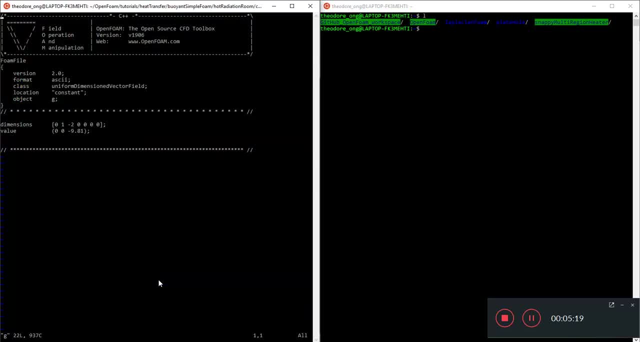 so we can take a look at G. this is a different G. this time this is a gravity 9.81. we can take a look at turbulence properties. so this is a K-Epsilon model, very basic turbulence model. nothing too fancy, it's just. if you're not familiar, please go and take a look at my. 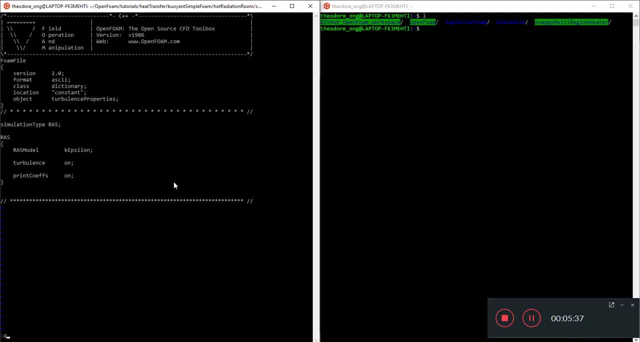 intermediate open form course where I'll talk through some of turbulence. take a look at the thermal physical properties and since we are kind of a little more into boy and simple form, we can explain these things a little more in detail. alright, so what is H-E, rho thermal? what is all this talking about? 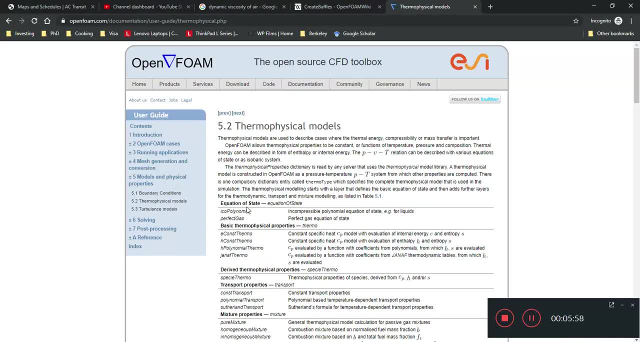 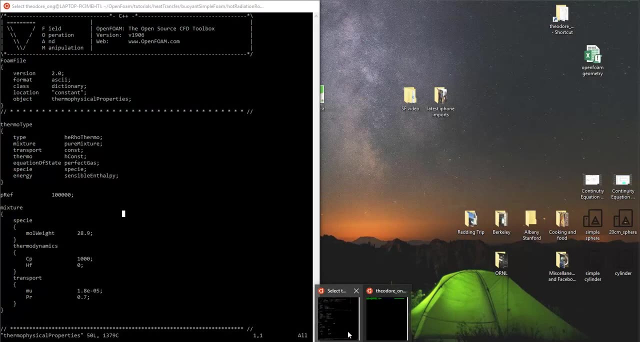 this is, on the side here called thermal physical models. so open form can allow thermal physical properties to be constant or a function of temperature, pressure and composition. so basically, you have an ideal gas equation of state where there's a variable density. so what is this? 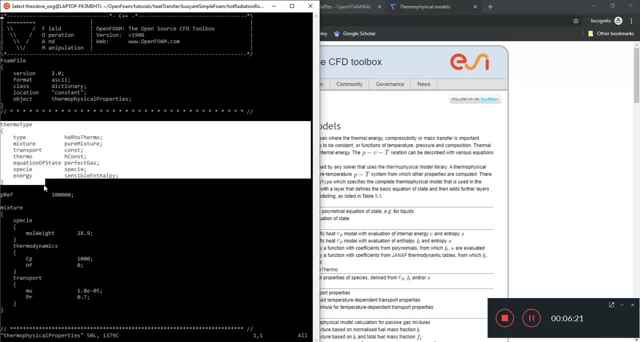 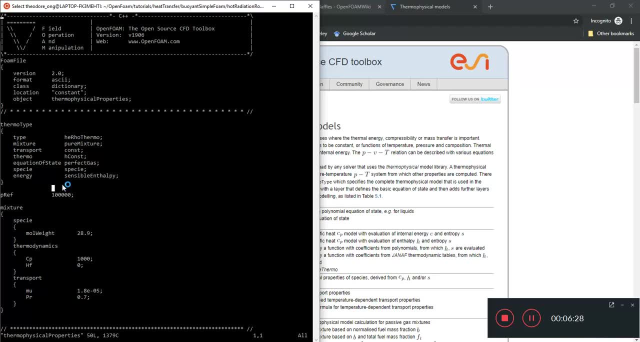 this is a thermodynamic package. how is this pressure-volume and pressure-specific volume, or in other words, density 1 over density? how is it all being calculated? so this is what is being used to calculate. so then you have some reference pressure down here. 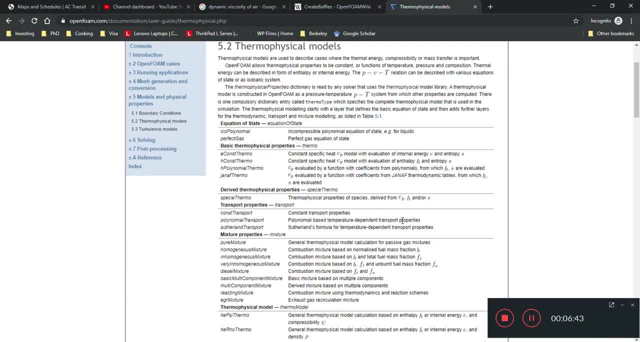 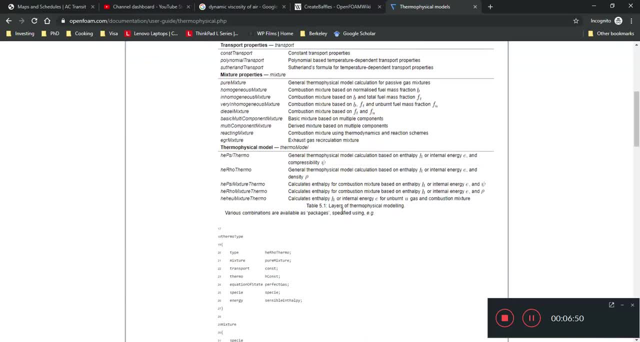 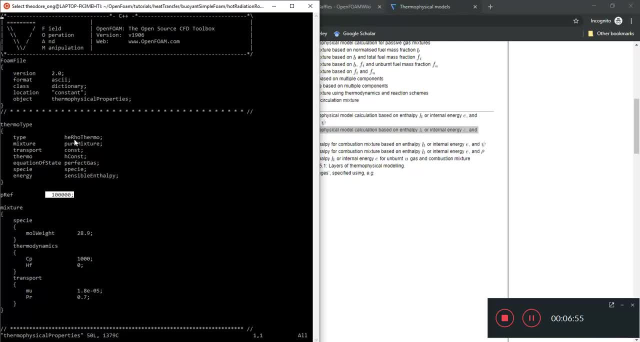 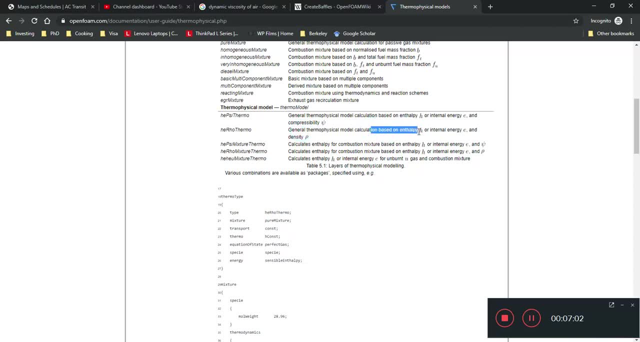 H-E rho thermal, which you can see over here. alright, H-E rho thermal. this is a general thermal physical model and the calculation is based on enthalpy, ok, or internal energy and the density. so that's why you have a H, which is enthalpy. 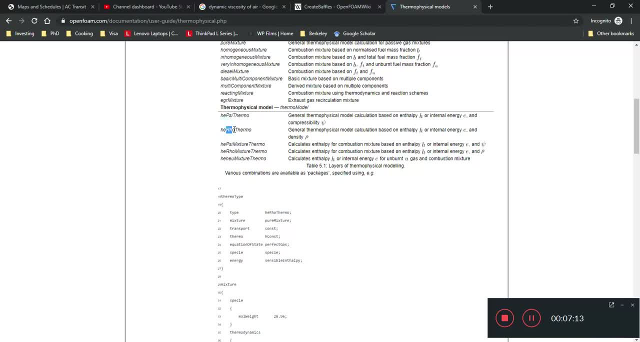 E, which is internal energy, and rho, which is the density. so this is what is used to calculate. now, of course, you can have other kinds of things here, for example H-E, psi, thermal- this one at this time of making this video. 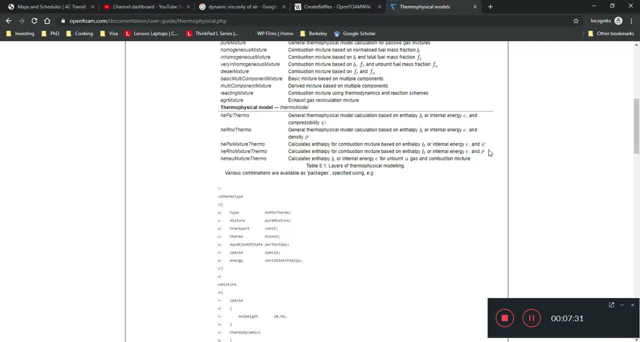 I'm not that sure what the psi is. I'll have to look that up, but in terms of this you can take a look. so this is, for example, a pure mixture. if you have a mixture, a pure, unchanging mixture, you can almost treat it as one homogeneous. 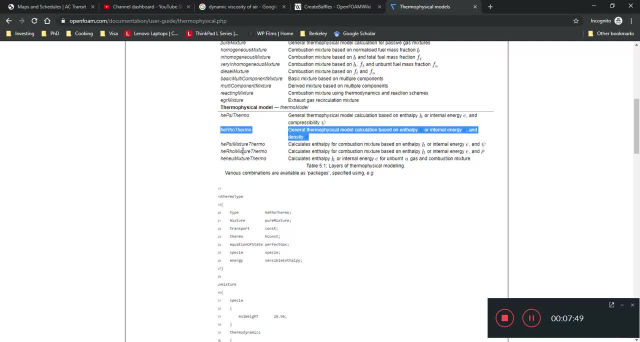 you can almost treat it as one homogeneous mix where the composition doesn't really change much. but let's say the composition changed, for example in this H-E rho mixture thermal, and you'll calculate enthalpy for combustion based on enthalpy H. blah, blah, blah. 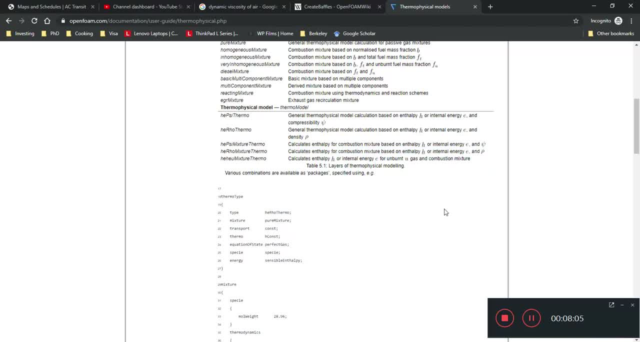 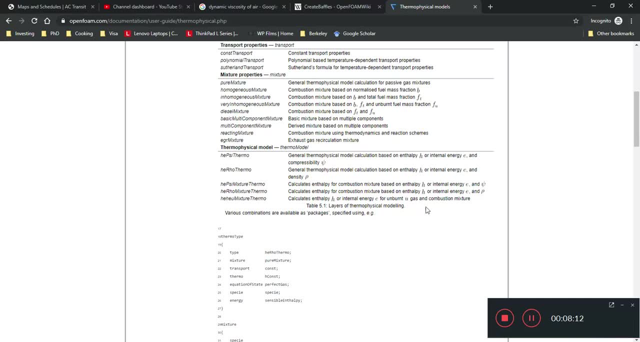 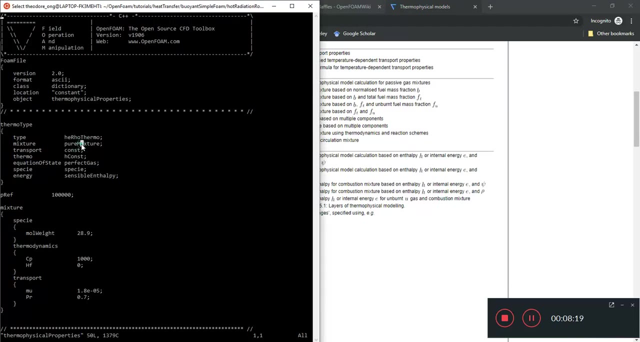 so this is for something where a chemical reaction is happening. an open phone can deal with that to give you the desired results. but in terms of heat transfer we are not going to talk too much about that. let's take a look at pure mixture. pure mixture is here. 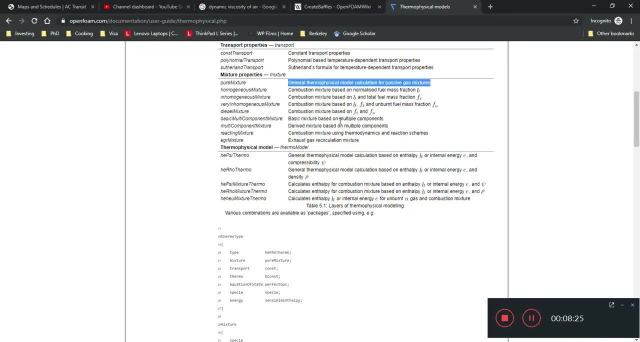 what is pure mixture? this one is a general thermophysical model calculation for passive gas mixtures. so for unreacting gas mixtures like air, you use pure mixture, which kind of makes sense. so transport, let's take a look at what the transport is saying. 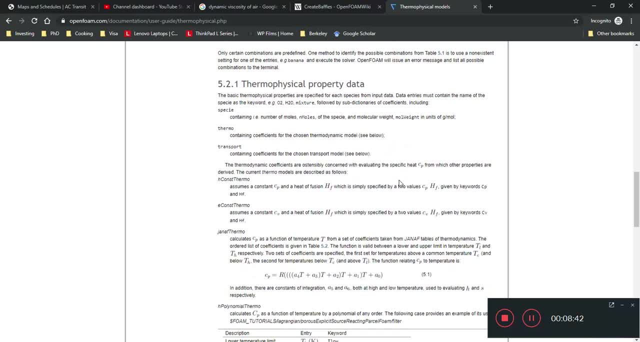 transport. it says it contains coefficients for the chosen transport model C below. so what is this chosen transport model? it says the thermodynamic coefficients are austen. okay, I'm not going to read that. I don't feel like it today, never mind. okay, so they are concerned with evaluating the specific heat. 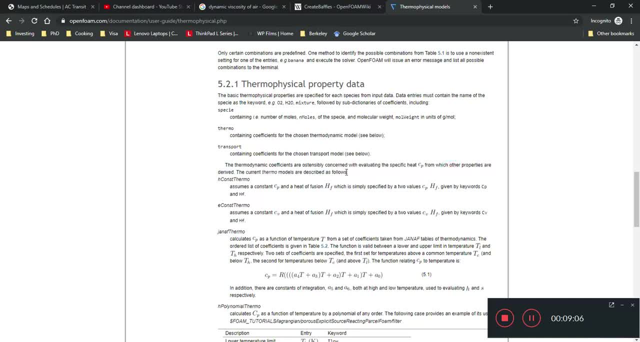 for which other properties are derived. the current thermal models are described as follows: H- constant thermal, which assumes a constant Cp- specific heat capacity. constant pressure, specific heat capacity. so Hf is heat of fusion and it's simply specified by two values, Cp and Hf, given by keywords Cp and Hf. 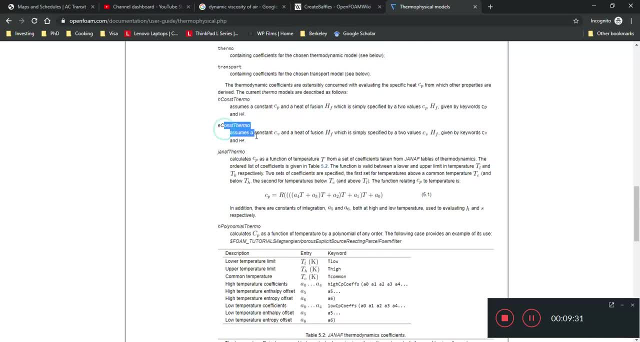 alright, there's the E constant thermal, which assumes a constant, constant volume, heat capacity and heat of fusion, and then this will be used to calculate. this is Jena or Yana, I don't know how to pronounce, but it gets Cp as a function of temperature, which is the so-called real. 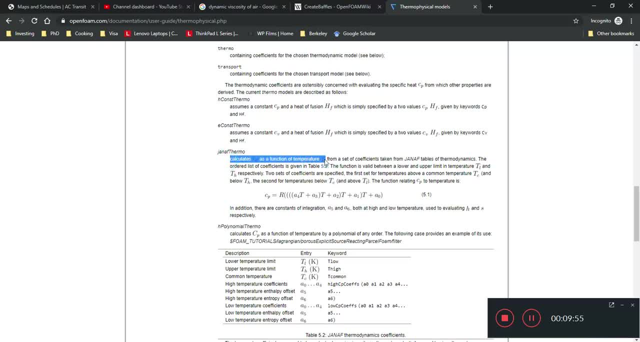 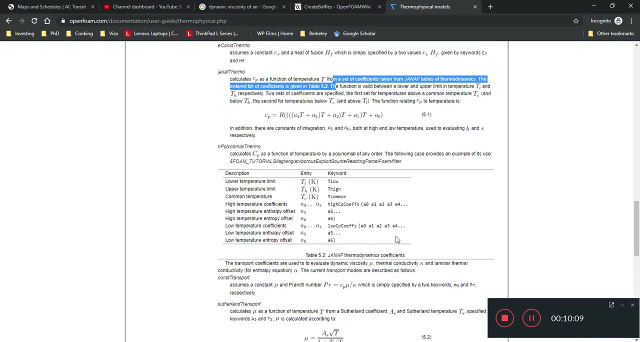 more real representation of what the constant value, the heat capacity, is like. so it gets it from some table of thermodynamics and the ordered list of coefficients is given in table 5.2. so this is how we define it. so, alright, these are the coefficients in table 5.2. 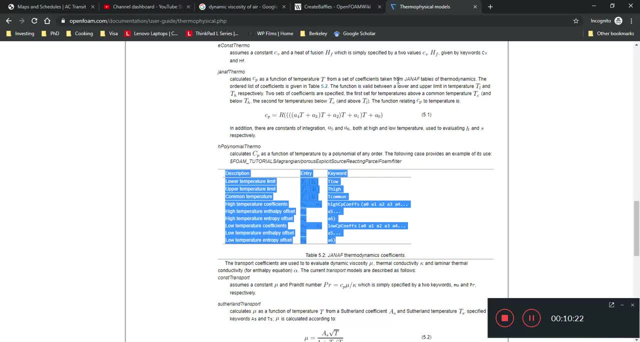 that's according to this guide. so you need to have a function between a lower temperature and upper temperature, as you have seen. especially chemical engineers, you should be familiar with this because you see this happening in Perry's chemical engineering handbook- pretty common. it's a varying Cp with respect to time. 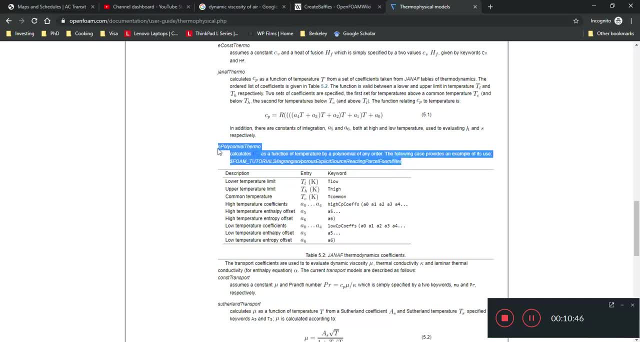 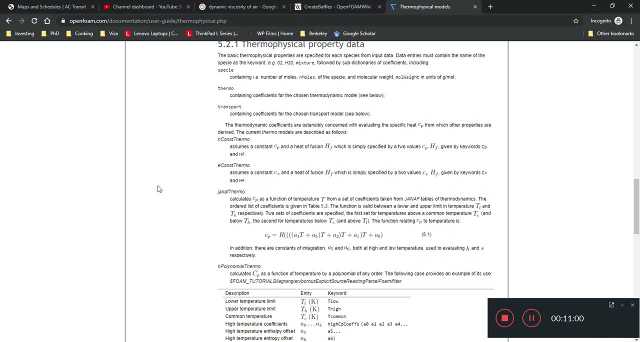 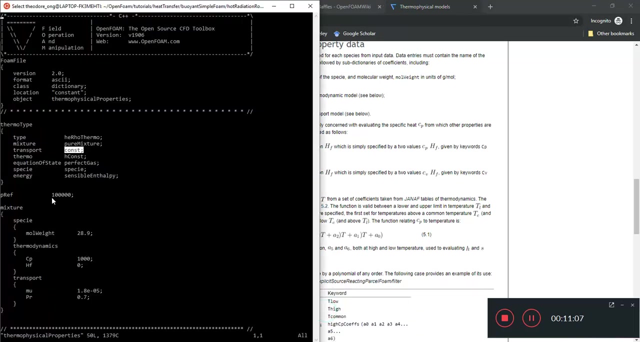 so if you want to have your own polynomial expression of the Cp, you can. you can actually give it as such. ok, so yeah, so transport model: ok, so let's take a look back here. thermal- ok, I think I was explaining for this one by accident. ok, so thermal is H constant. 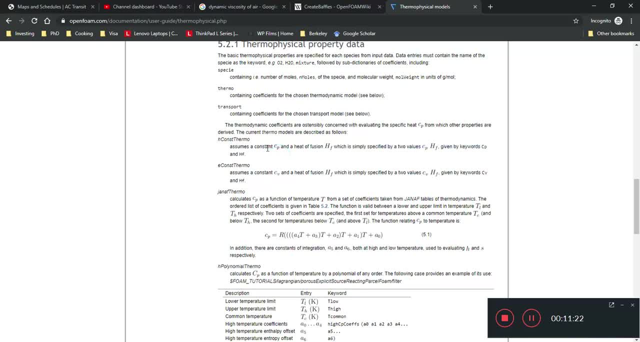 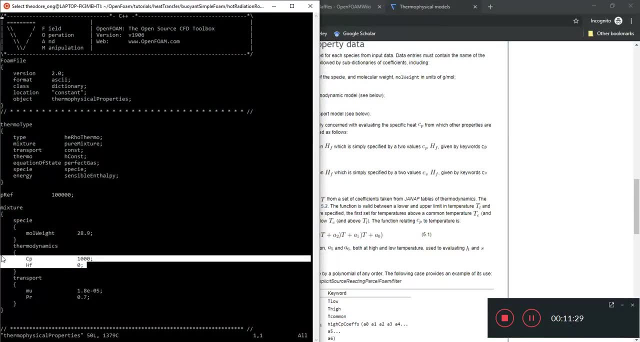 so this is very simple model. you just give two constants: one is Cp, one is heat of fusion. so I mean, at the temperature of our interest we have a constant pressure. specific heat capacity. heat of fusion is just 0 because there's like no phase change or anything. 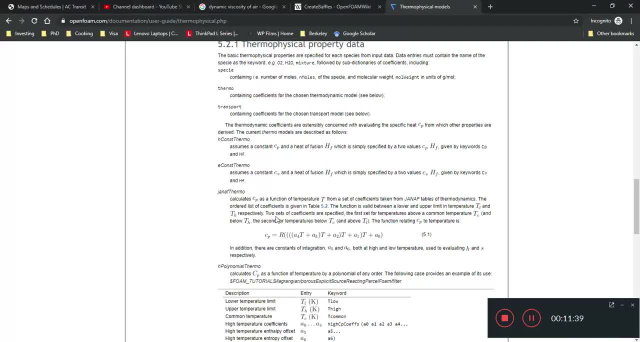 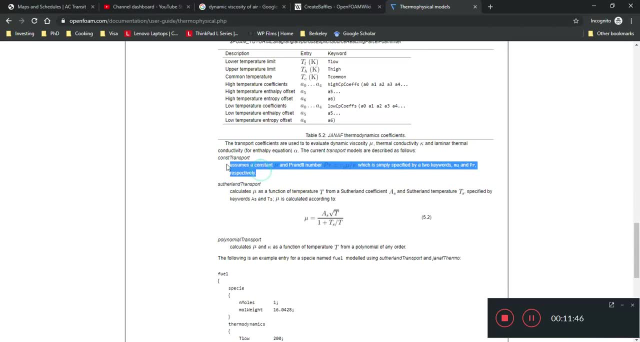 so you don't really have to bother, ok? hmm, so let's take a look at transport models. so what is this transport model? constant transport assumes a constant mu, which is a thermodynamic dynamic viscosity, and a Prandtl number, which is simply defined by two keywords. 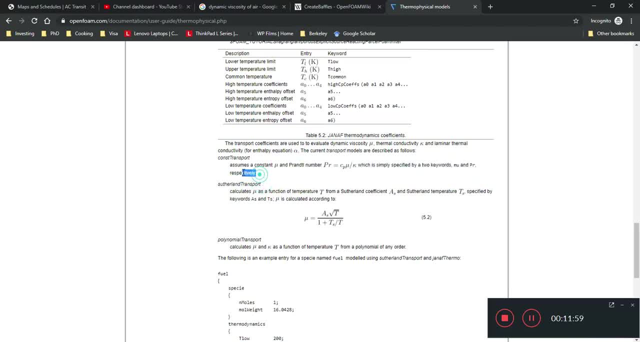 mu and Prandtl number. so this is the mass transport. mass transport, I think, oh yeah, because it talks about viscosity, it talks about convection, so that will affect convection a lot and the heat transfer, of course. so it assumes a constant dynamic viscosity and Prandtl number. 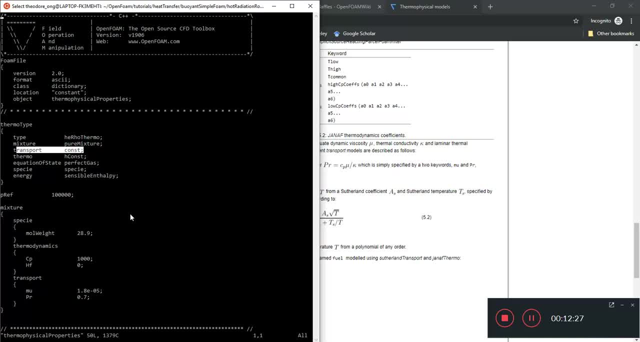 so this is what the transport model is talking about. so you can see. for, let's say, thermodynamics, you have to define the Cp and Hf for the transport, you have to define the mu and Prandtl number, so of course you can have other again. 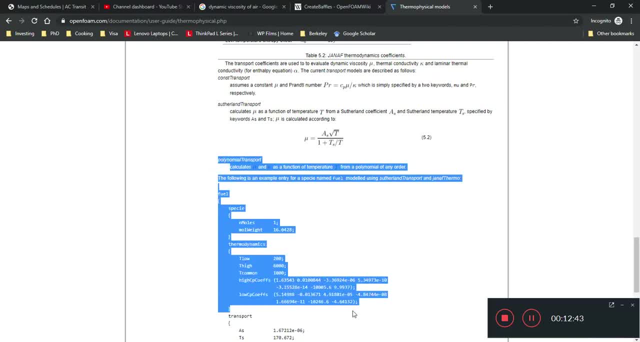 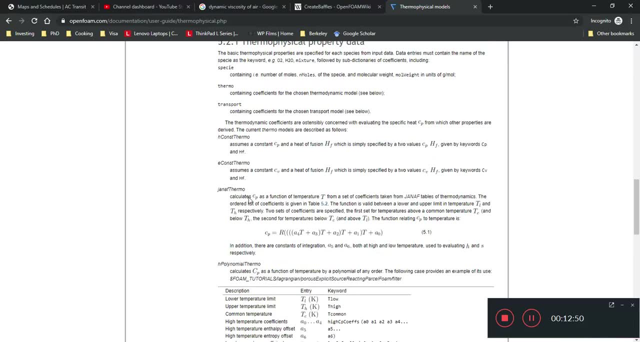 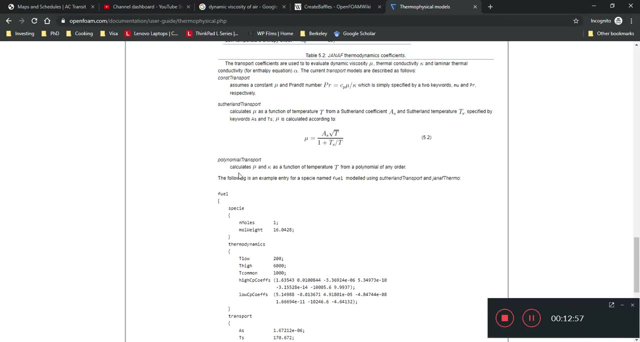 other polynomial functions. as before, as much as you can calculate thermodynamics properties such as Cp based on temperature, you can define mu and Kappa, which is the. this is part of Prandtl number anyway. you can define this as part of a temperature function, which is again more realistic. but 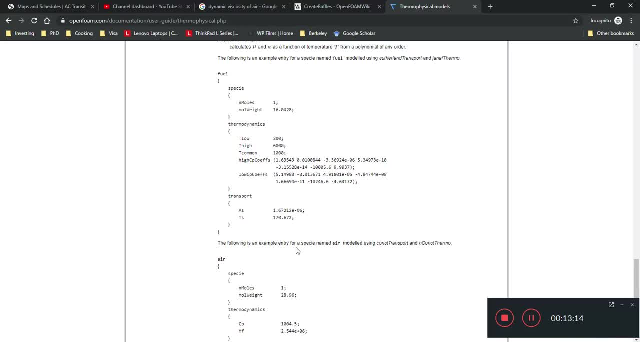 it is more realistic, but doesn't really. you don't really need that complex a model for air. so in this case air will look something like that. so there's a species named air and the species is like some number of moles. molecular weight, thermodynamics and transport are listed here. 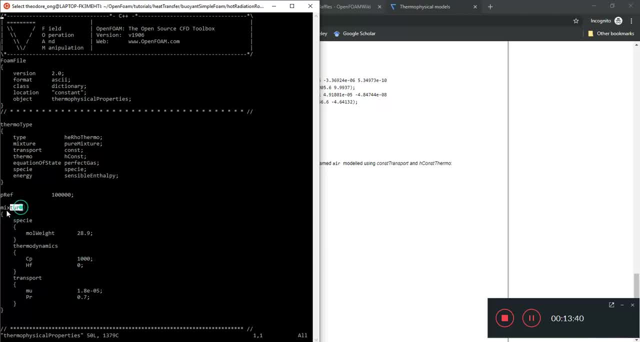 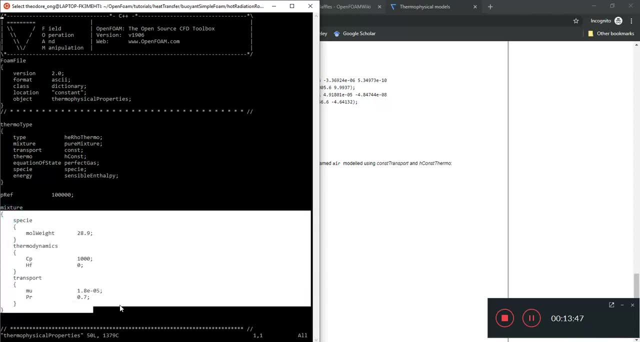 so in our input file we just name it as mixture, name it as mixture, and the species is this, which is obviously air. we just don't call it air. but that's that. let's go through the other options. we'll explain it bit by bit. equation of state. 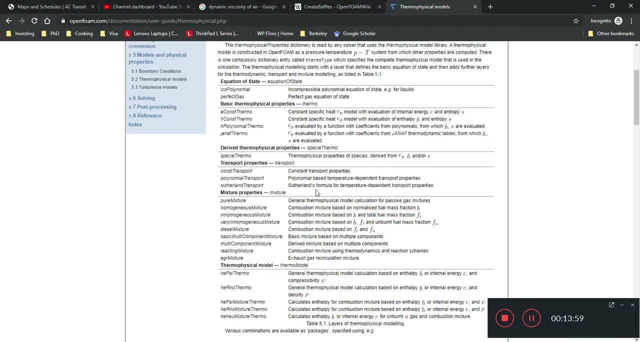 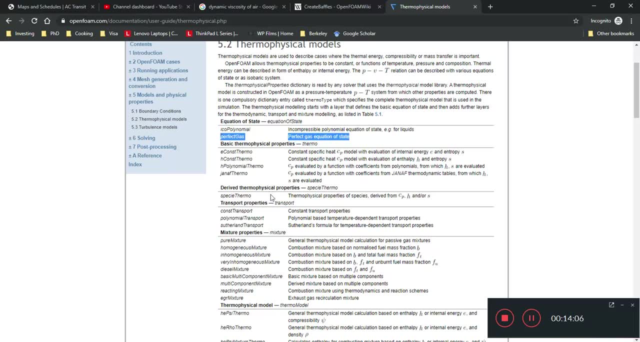 this one's fairly simple. let's see whether we can find other equation of states here. alright, so you have a perfect guess here. perfect guess equation of state, or ideal guess. pv equals nrt, or icopolynomial, which is an incompressible polynomial equation of state. 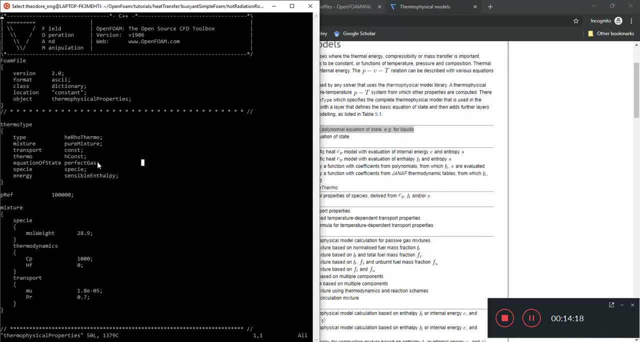 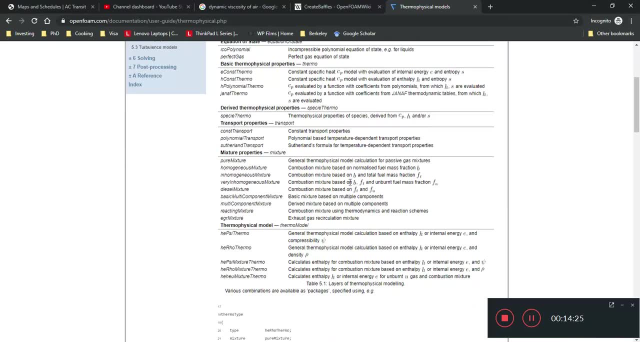 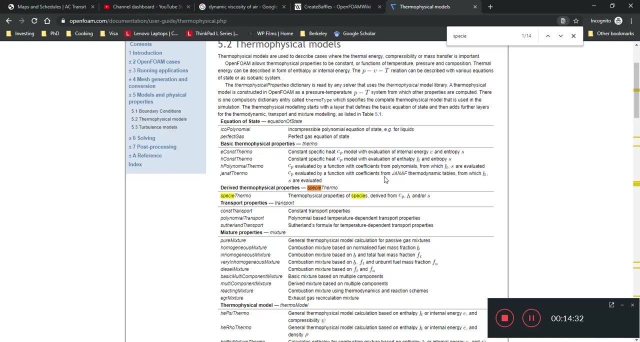 for example, for liquids. okay, so in this case the equation of state is a perfect guess. liquids- okay, so I believe there is one thing called specie s-p-e-i-c-e. alright, okay, so this is derived thermal physical properties. so this says that thermal physical properties 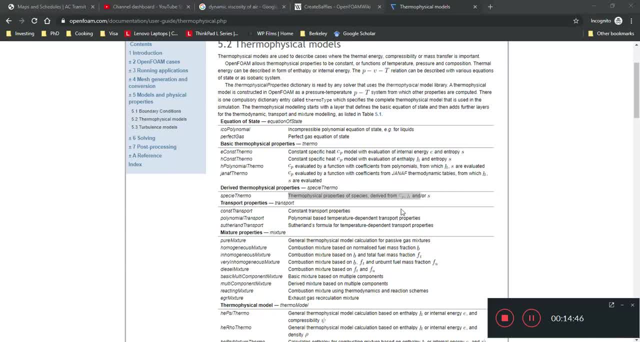 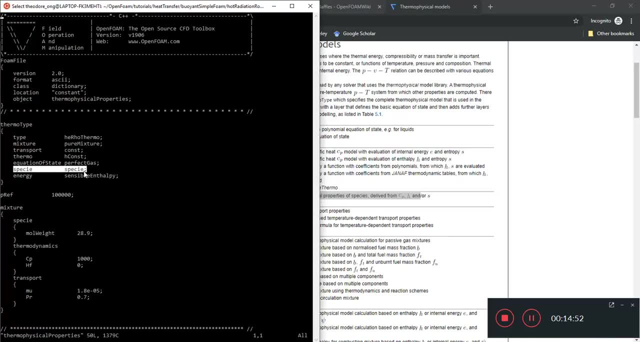 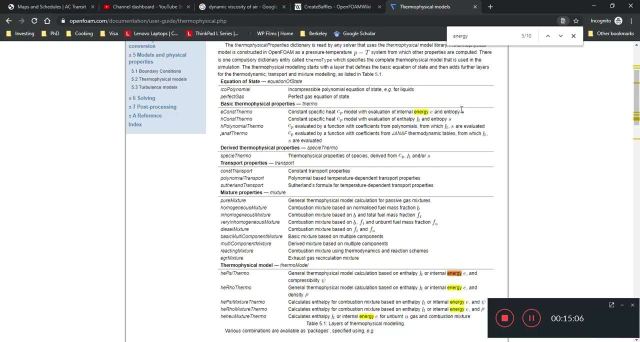 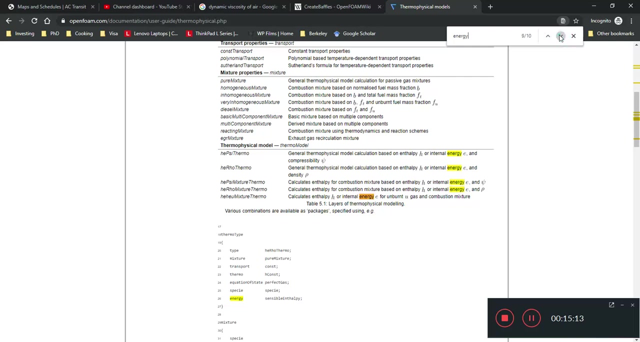 are based on c-p-h-n-r-s. so I suppose, yeah, you have to. what this is saying is that, okay, based on these two, based on this thermodynamic model, you calculate everything else. so that is that let's go for energy, for the energy entry, alright, so